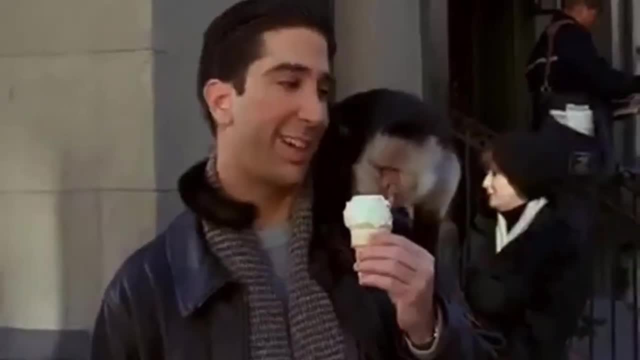 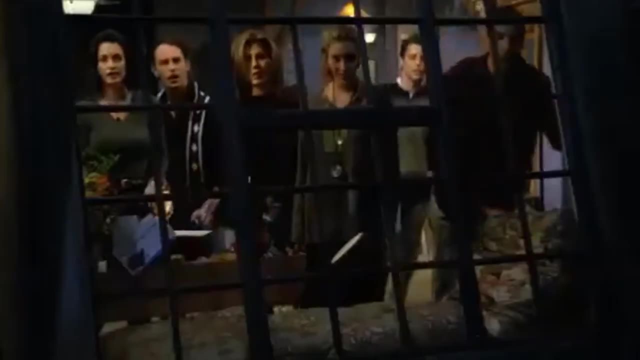 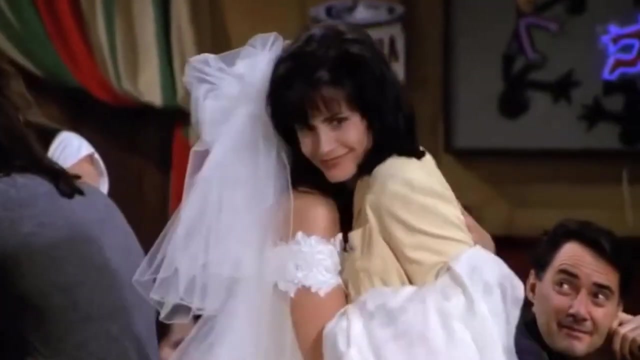 lives. The show first aired in 1994 and lasted 10 seasons, with the cast growing in popularity as the show progressed. Friends had a budget of 10 million dollars per episode in the last few seasons because the cast had become well known and their pay reflected this, resulting in a higher 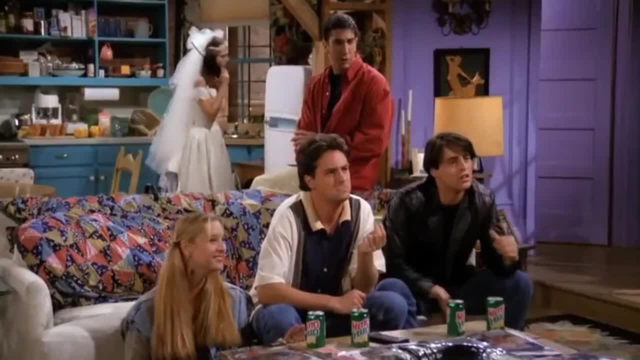 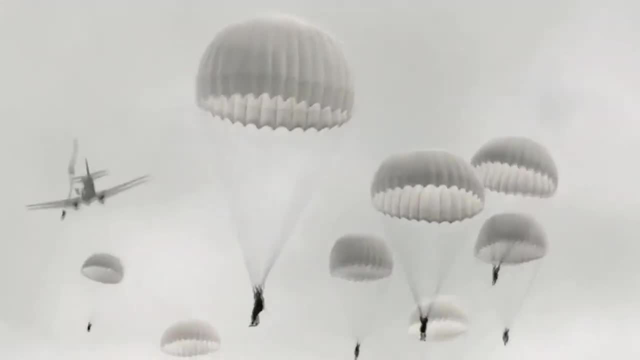 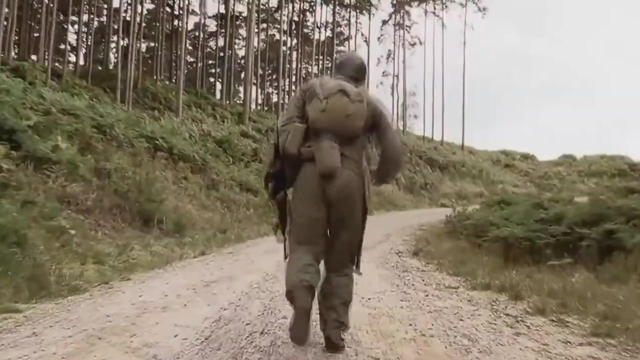 budget. Making Friends, one of the few sitcoms with such a large budget. Number 9. Band of Brothers: 12.5 million dollars per episode. Created by Tom Hanks and Steven Spielberg, Band of Brothers is one of the highest rated and most expensive television shows ever. 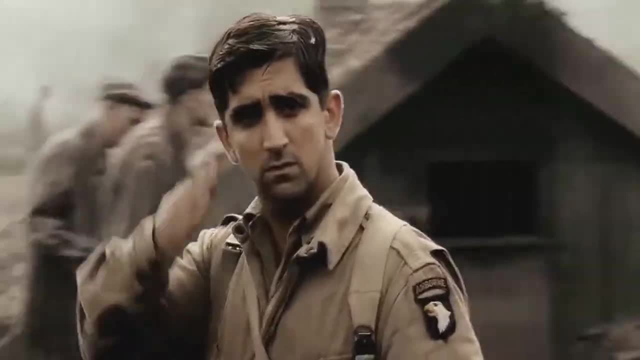 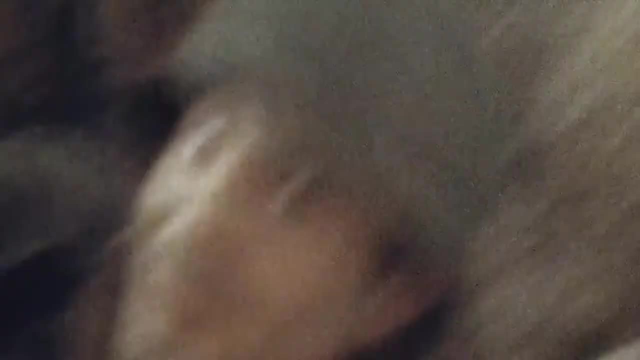 When the first show aired in 2001,. a budget this large for a tv series was unheard of, but HBO approved the project because it was overseen by big names like Tom Hanks and Steven Spielberg. Number 8.. ER 13 million dollars per episode. 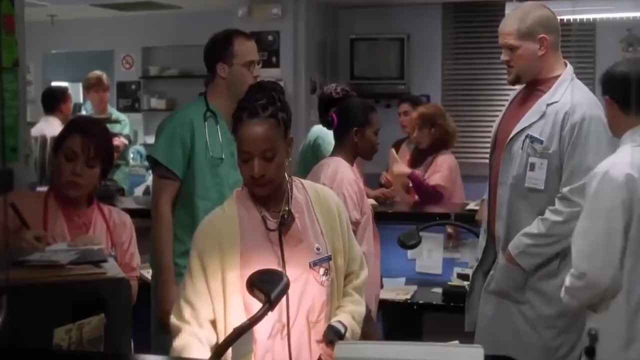 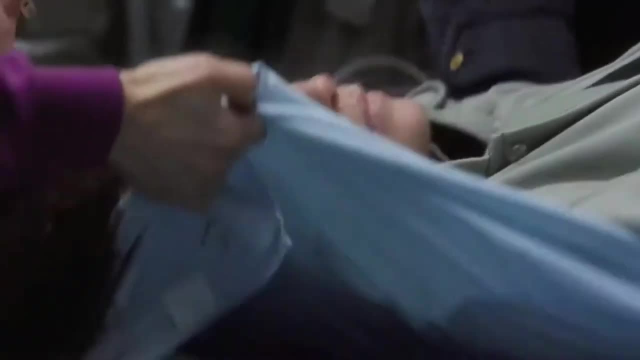 On the surface, ER appears to be a typical medical drama, but during its heyday in the 1990s, it was one of the most influential and popular shows of all time. Many current Hollywood stars, including George Clooney, have benefited from the series, which was created by Jurassic. 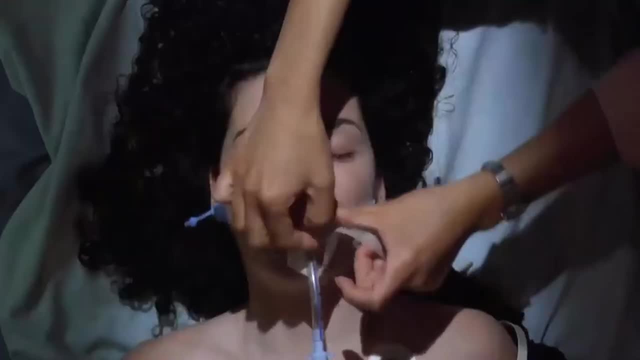 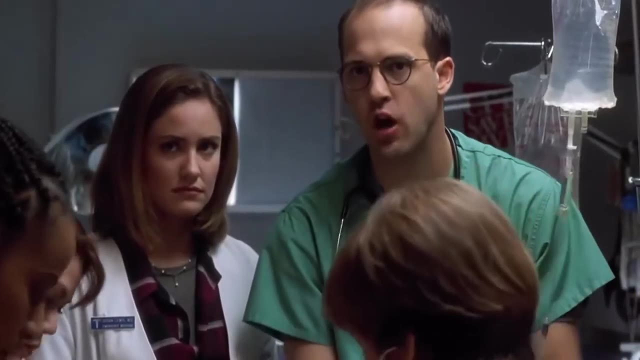 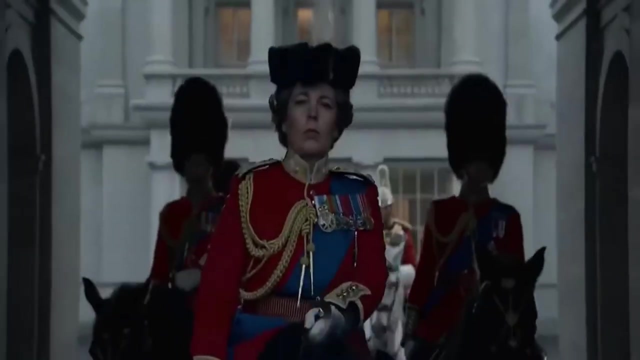 Park writer Michael Crichton. Although the show's initial costs were reasonable, the show runners were so desperate to keep Clooney in the cast that they agreed to such extravagant budgets during his peak popularity. Number 7. The Crown: 13 million dollars per episode. 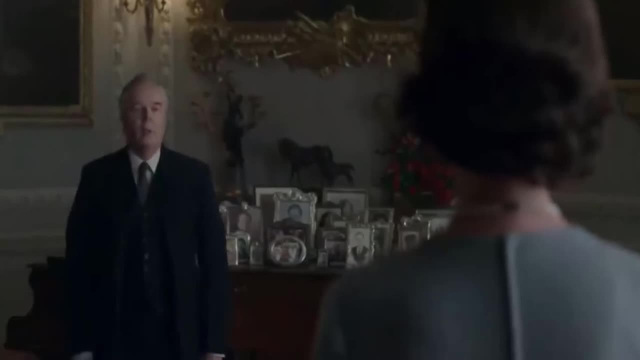 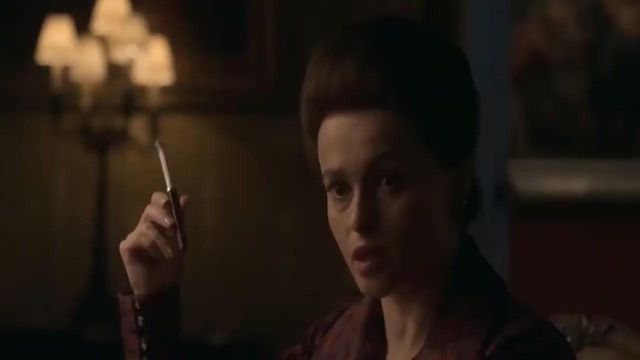 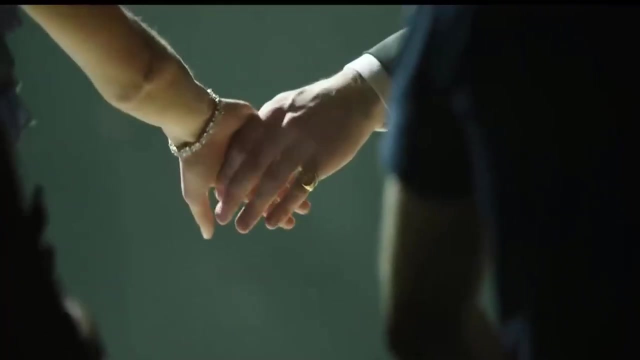 The Crown is one of, if not the most expensive, Netflix series ever. The series follows the life of Elizabeth II from her childhood to her current reign. The lavish recreations of historical events and royal aesthetics consume a significant portion of the budget. The series' meticulous attention to 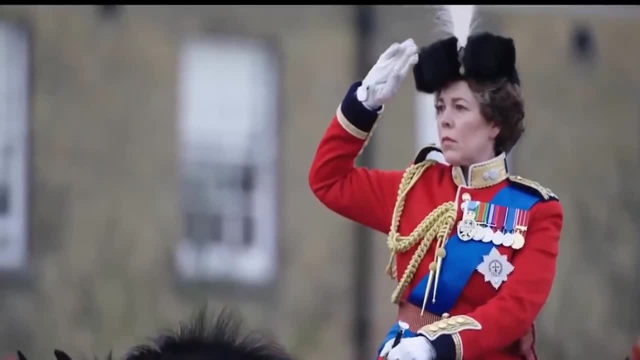 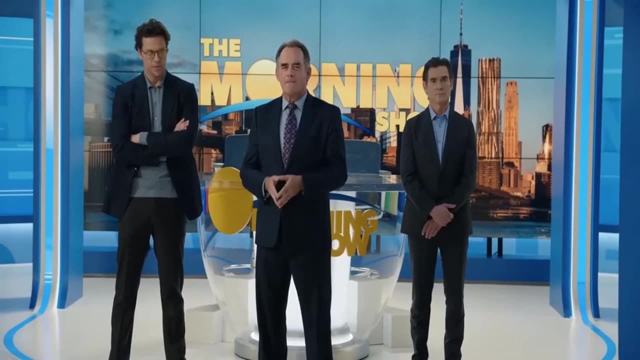 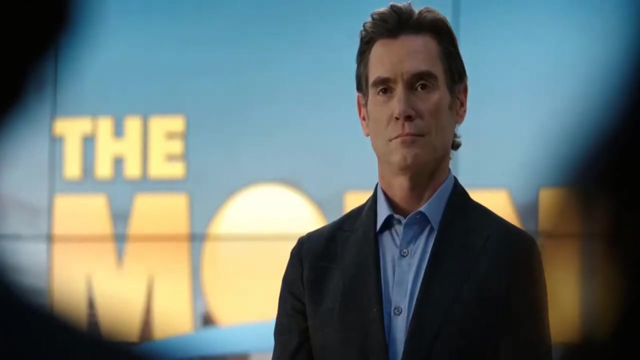 detail has earned it a well-deserved reputation, but it comes at a price, Number 6.. The Morning Show: 15 million dollars per episode. Apple is known for investing indefinitely to provide quality to its customers at any cost, and the same principle is being applied to their. 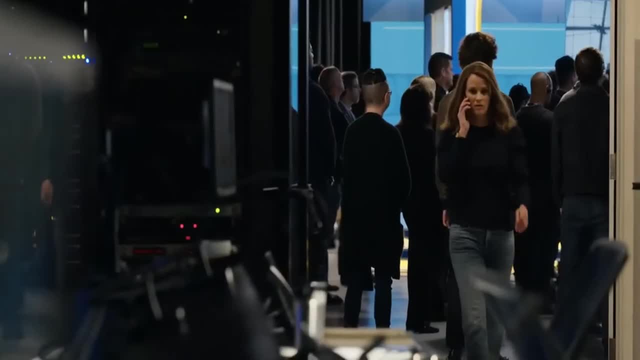 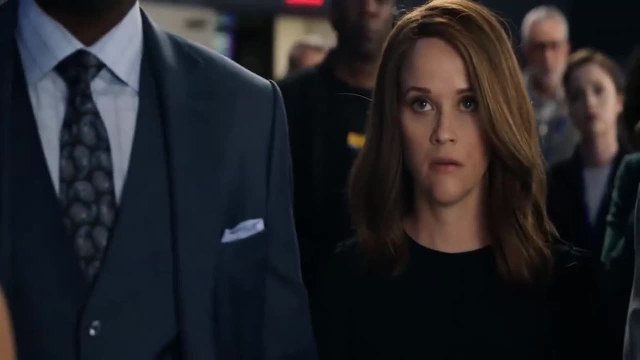 streaming service Apple TV+. They plan to invest 6 billion dollars in the production of TV shows and movies for their streaming service. according to reports, The salaries of the actors, including Jennifer Aniston, Reese Witherspoon and Steve Carell, consumed a large portion of the show's. 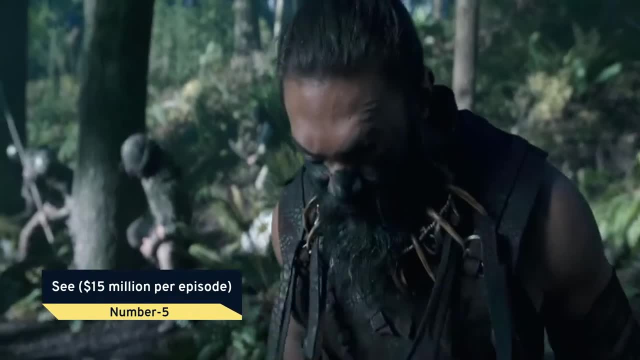 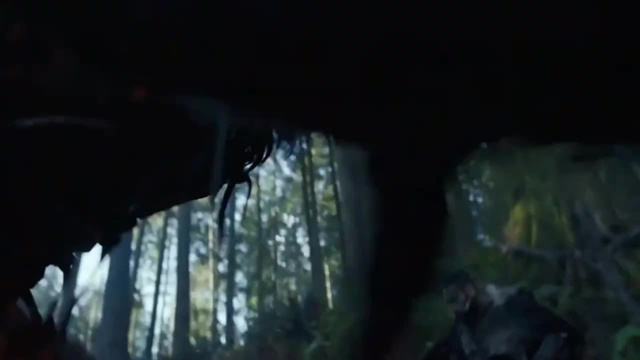 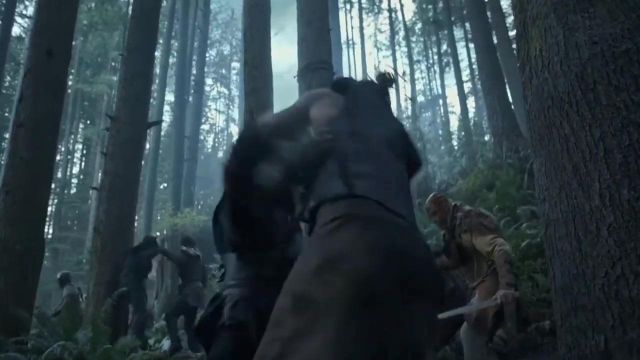 budget Number 5. Sea: 15 million dollars per episode. Sea, another Apple TV Plus series, has a similar budget to The Morning Show, but for different reasons. Jason Momoa stars as Baba Voss, the leader of a tribe in a world where humans have lost their 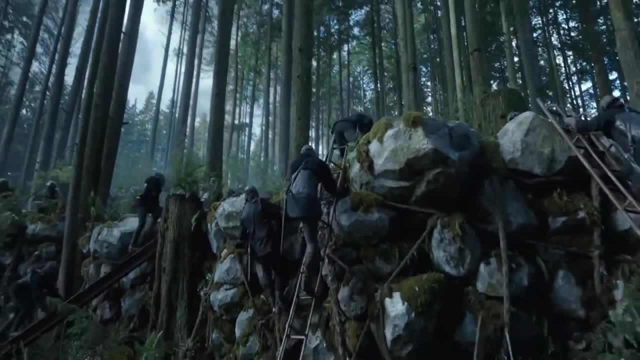 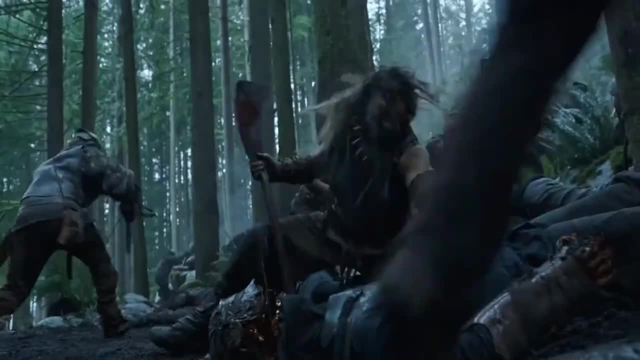 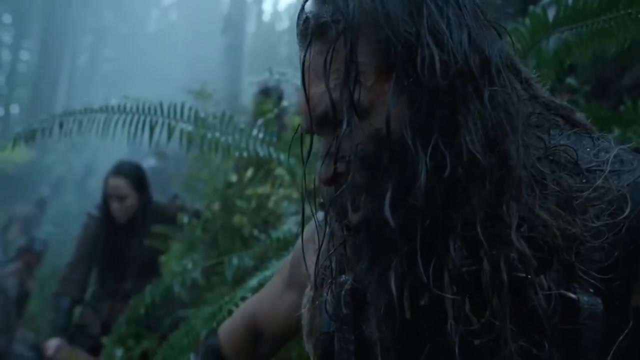 vision and have adapted to a different way of life for centuries: The birth of two visually impaired twins. the tribes are thrown into chaos as a result of this. The series, which is set in a dystopian future, makes extensive use of CGI, resulting in a final cost per episode of 15 million. 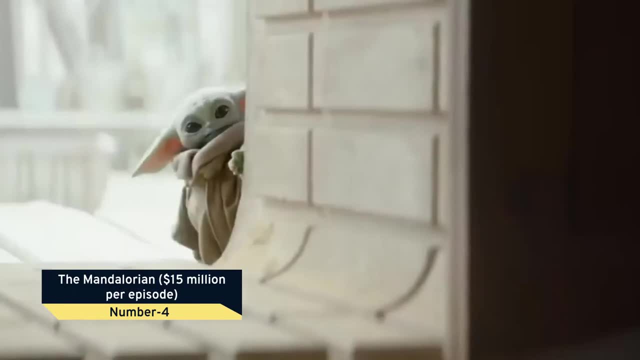 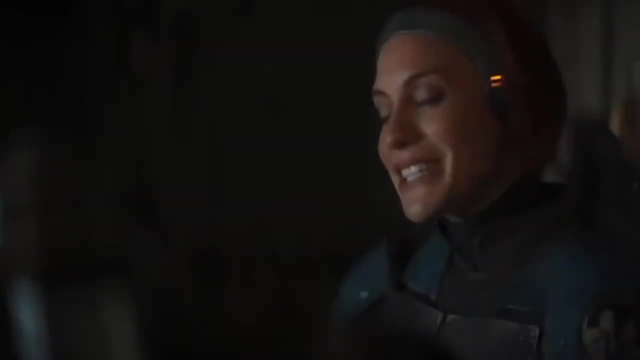 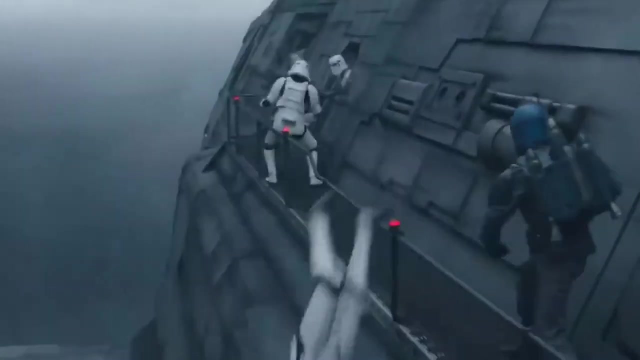 dollars. Number 4. The Mandalorian: 15 million dollars per episode. The Mandalorian, a Disney Plus original series created by Iron Man director Jon Favreau, was an instant hit when it debuted. The series had a lot of leeway in terms of plot and character. 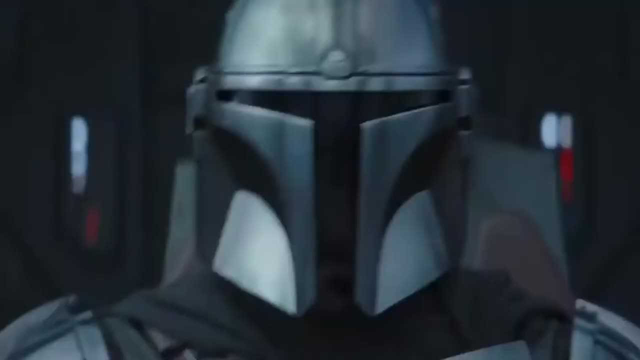 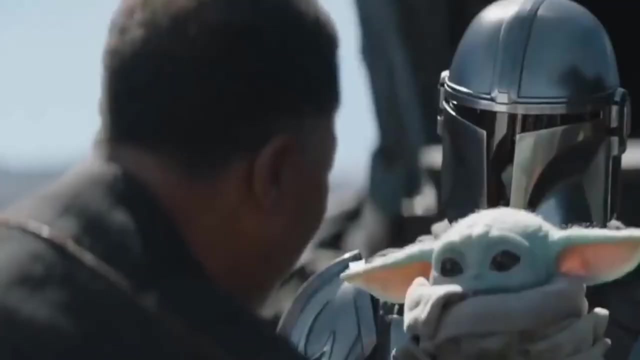 development because it took place in the Star Wars universe but was not directly connected to any of the mainstream films. Critics praised the actors' action and performances, especially Baby Yoda, who went viral on the internet. The space western features cutting-edge, practical and 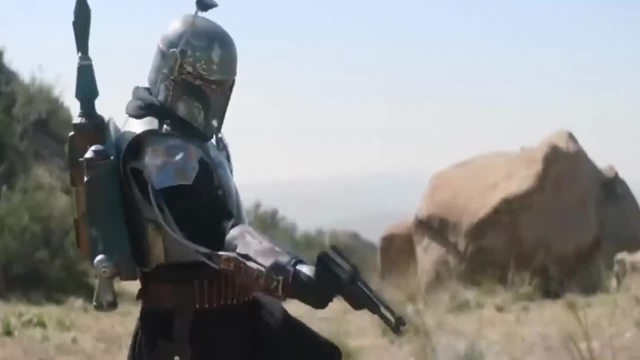 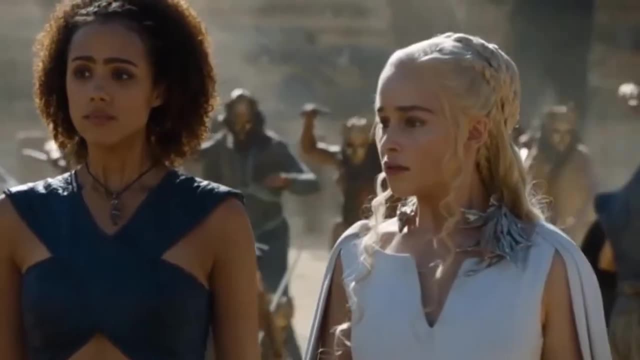 computer-generated animation, both of which are available on the Star Wars universe website. The effects: with the baby yoda puppet alone costing around 2 million dollars. number three: game of thrones: 15 million dollars per episode, it's no surprise that one of the most ambitious shows 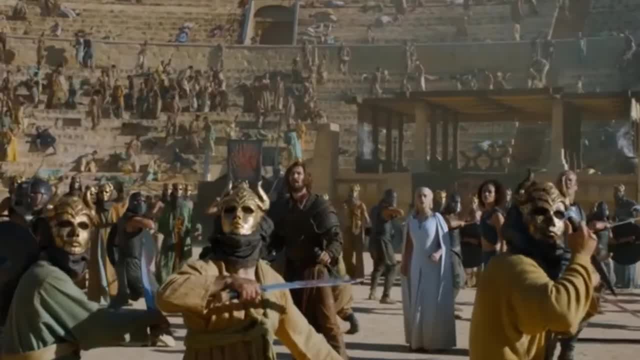 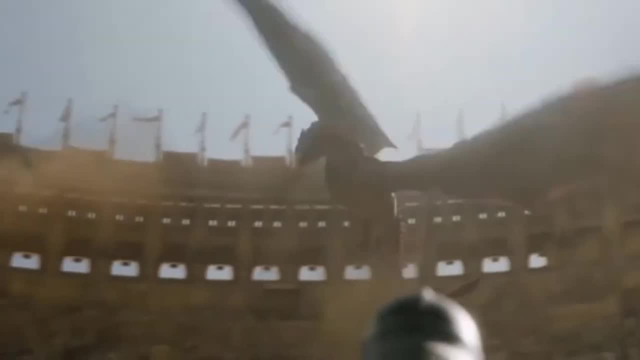 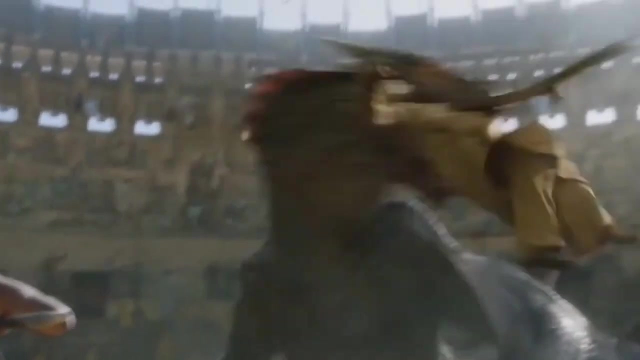 ever made the list. when hbo's game of thrones first aired in 2011, it captivated audiences around the world and it remained one of the most expensive and well-produced shows on television for many years: exotic locations, massive cgi and tons of special effects, not to mention the salary. 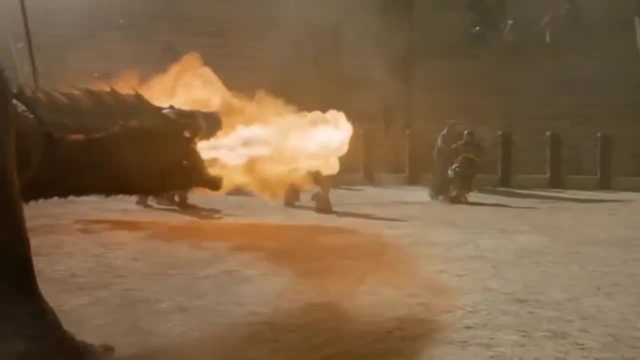 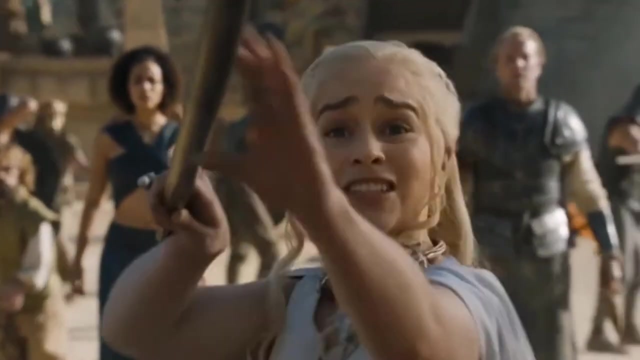 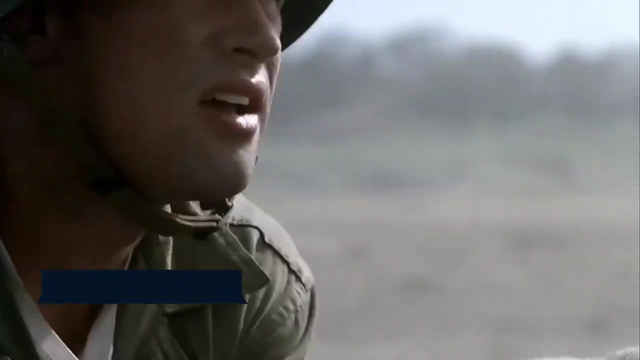 of the large cast all contributed to the cost increases. each episode cost at least 15 million dollars in the final season, which was slightly more expensive than the previous ones. despite the fact that previous seasons had not been this expensive, the difference was not significant. number two: the pacific: 20 million dollars per episode. 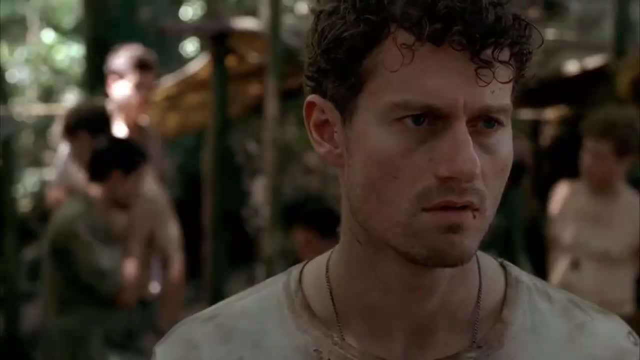 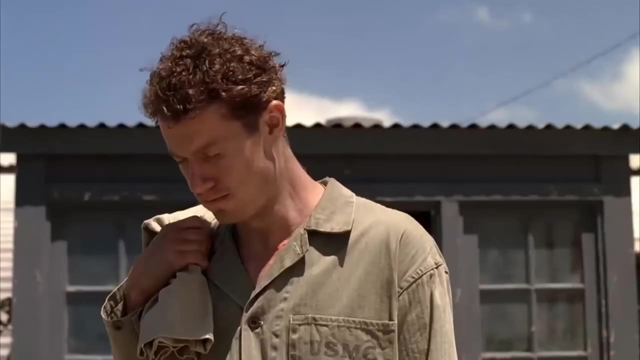 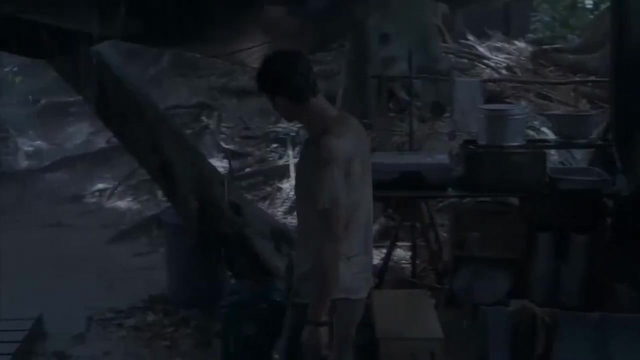 hbo's the pacific, which premiered in 2010, is still the most expensive limited tv series the network has ever produced. producer steven spielberg and tom hanks didn't cut any corners when it came to recreating some of world war ii's bloodiest and most violent battles. the budget for